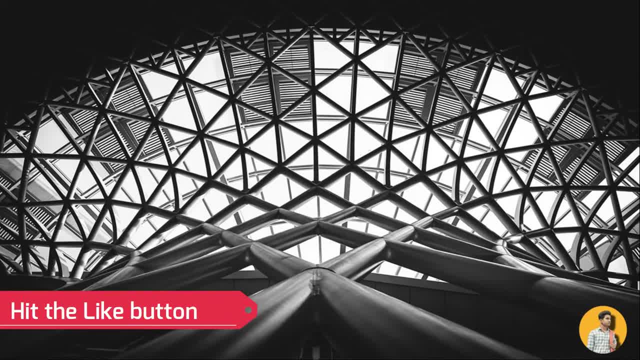 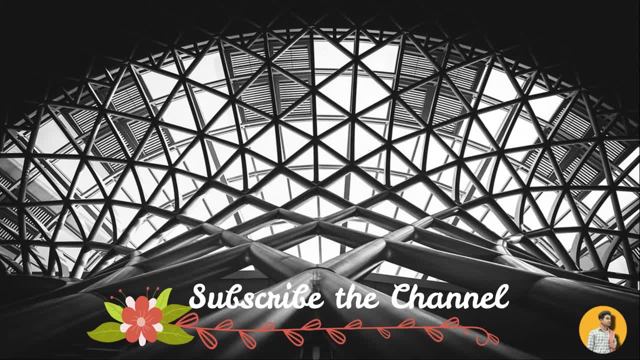 In the same way, the architecture is a domain that majorly deals with geometry and visuals. It plays a visual role in design as well as construction. Geometry was the only one used for over 2,000 years Now. there are many different aspects developed with time. 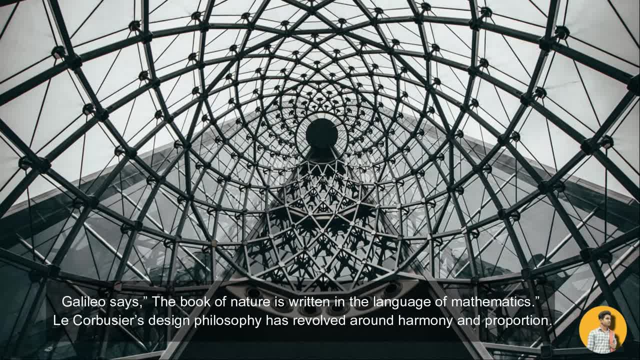 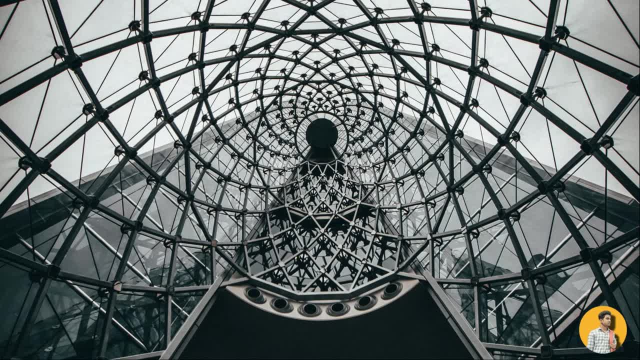 Galileo says the book of nature is written in the language of mathematics. Le Corbusier's design philosophy has revolved around harmony and proportion. These rhythmic patterns are inventively seen in human activities. Hence he developed an anthropometric system of modular which goes by principles of golden ratio. 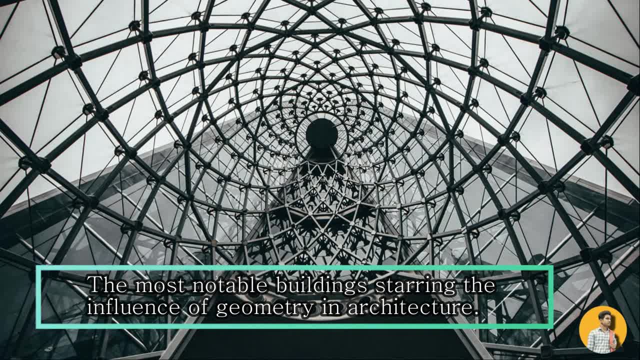 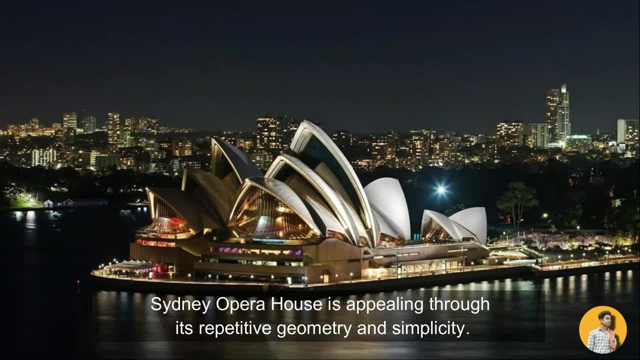 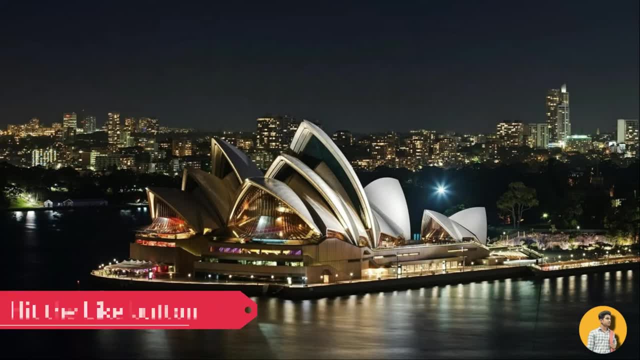 Let's discuss the most notable buildings starring the influence of geometry in architecture. First is Sydney Opera House at Australia. Sydney Opera House is an appealing through its prospective, geometry and simplicity. The roof design evolved from parabolic ellipse, solid, to finely spherical geometry for the final forms of the building shades. 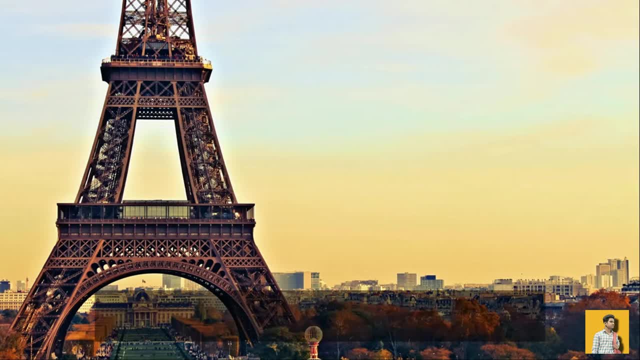 Second is Eiffel Tower at Paris, France. With hundreds of triangles and parallelograms, Eiffel Tower is one of the ideal examples of geometry and technology. A pyramid-like geometric shape on four sides with large half-circles on each other side is a design wonder. 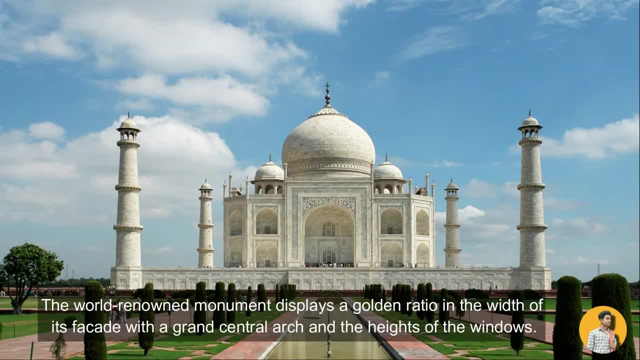 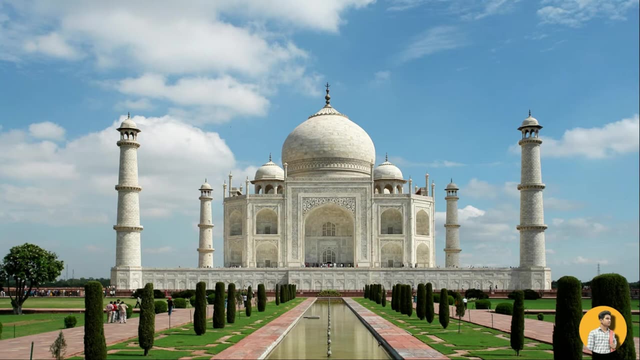 The third one is the Taj Mahal at Agra, India. The world-renowned monument displays a golden ratio in the width of its façade, with a grand central arch, and the heights of the windows. Mughal architecture has a particular mathematical order and an astounding aesthetic, with perfect symmetry and harmony. 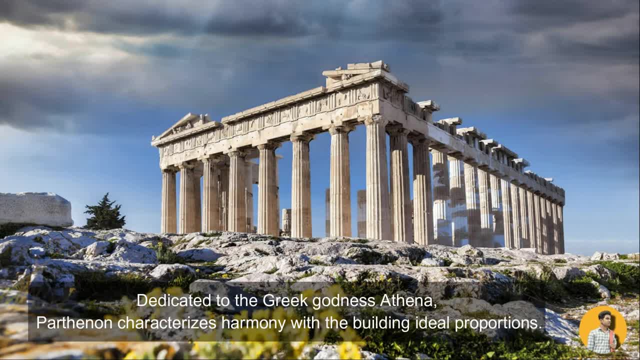 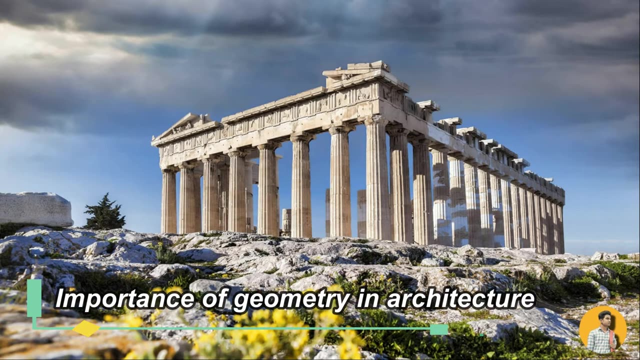 Fourth is Parthenon at Greece, dedicated to the Greek goddess Athena. Parthenon characterizes harmony with the building ideal proportions, The ninth ratio, 4, with the height ratio. despite the vertical and horizontal proportions, The element of its façade can be seen symbolizing golden triangles. 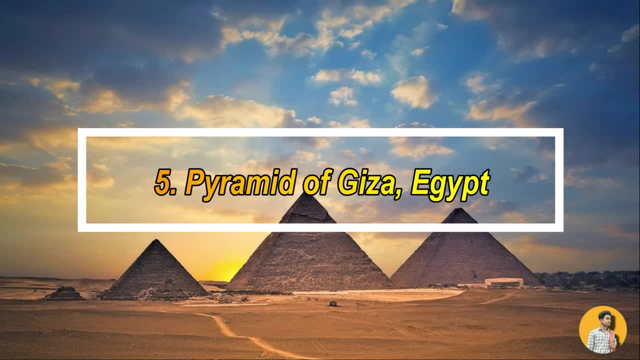 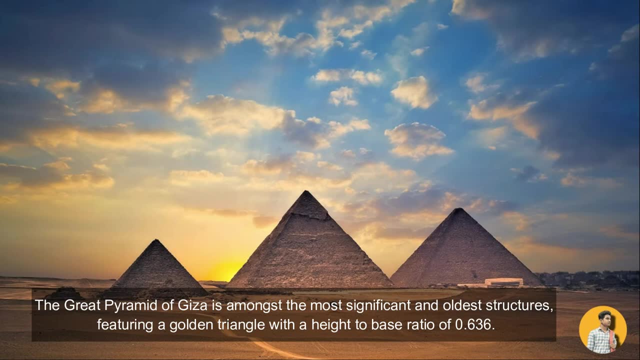 Last but not the least, the fifth one is the Pyramid of Giza at Egypt. The Great Pyramid of Giza is among the most significant and oldest structures, featuring a golden triangle with a height-to-base ratio of 2.5.. It has a height-to-base ratio of 0.636..